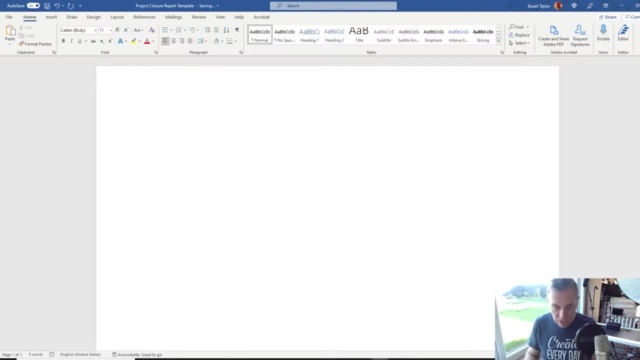 mobile devices can see clearly. Okay, let's get this cover page started. Just drop a few lines there, Go to styles and select title. We'll put project closure report And then we'll select a larger size font, Maybe a 20., And put here project name. Reduce the font slightly And then put project. 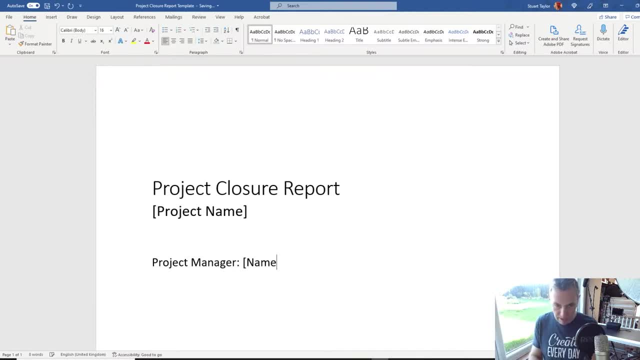 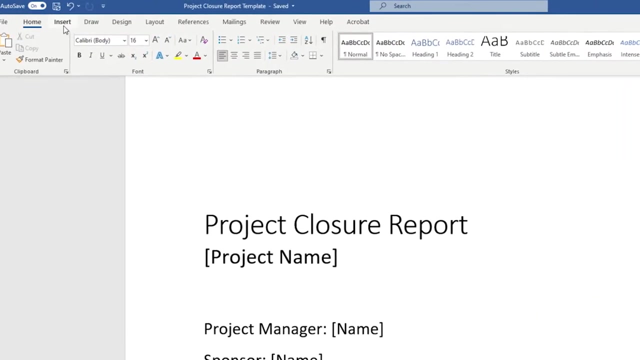 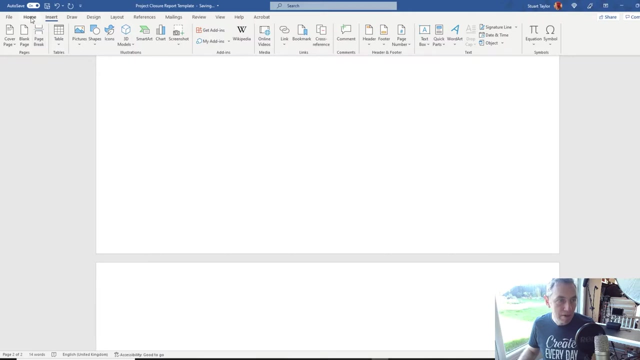 manager And put your name in the box. Sponsor, Put their name in the box And then we'll go to date of report And then put the date in whatever format is suitable to you And then we go to insert, Put a page break, And this is where we'll put our contents. page Go back. 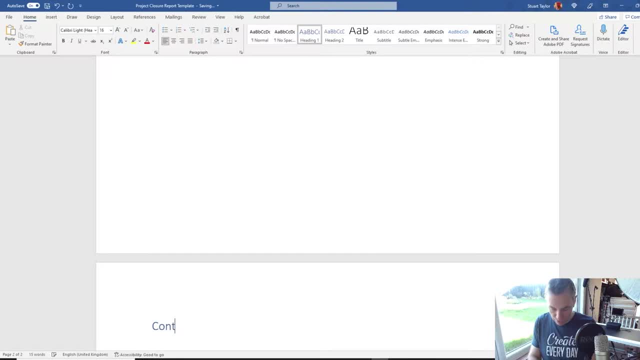 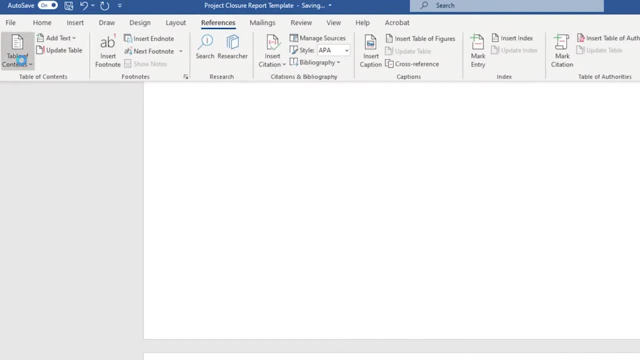 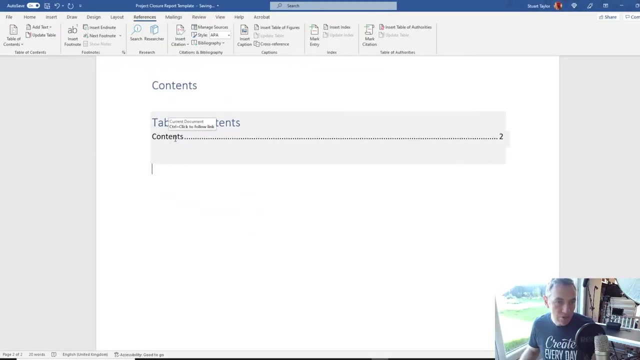 to home, Select heading one, All these contents, And then go to references, Select table of contents And pick any of these that you like. I'm going to go with automatic table two And you see it's already looked up the contents there because, if you recall, I used heading one. 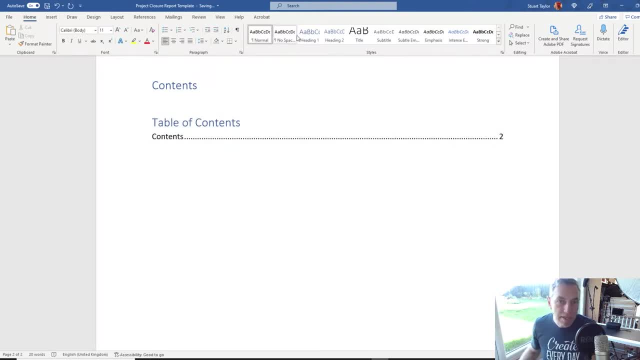 This is looking up headings Underneath the table of contents or on a separate page, if you prefer. we'll put a list of the reviewers on here, because you might have a situation where somebody has to sign off these documents and you might want to keep a list of who and 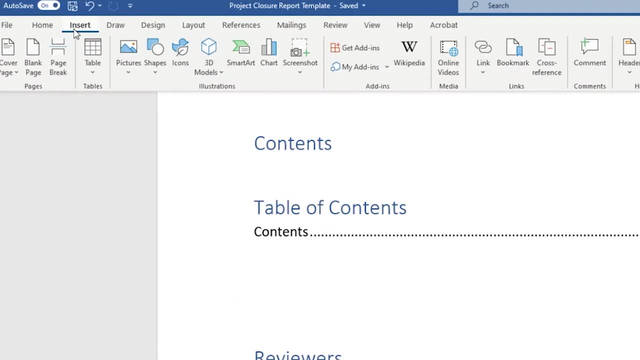 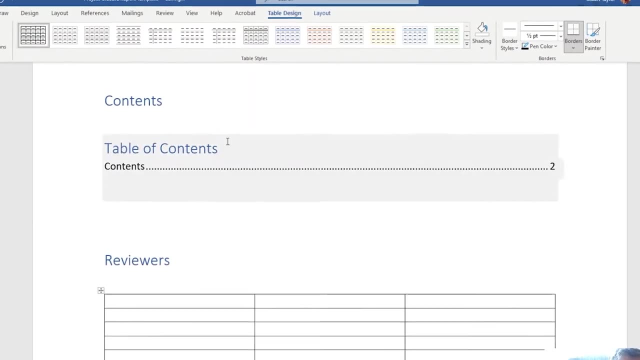 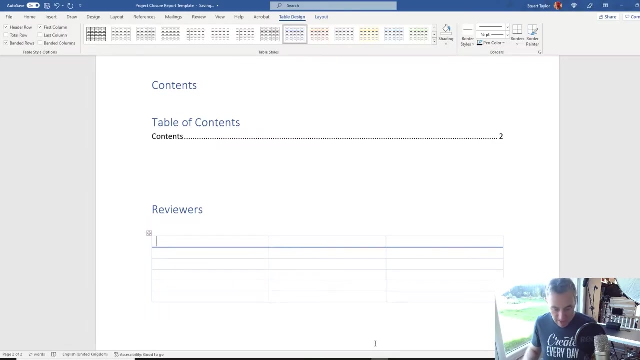 when they did that. OK, So let's do that. So let's show you how it works. And in the charts I'm going really quickly. what I'm going to do is just enter the name of your share. Here's my sentiments. 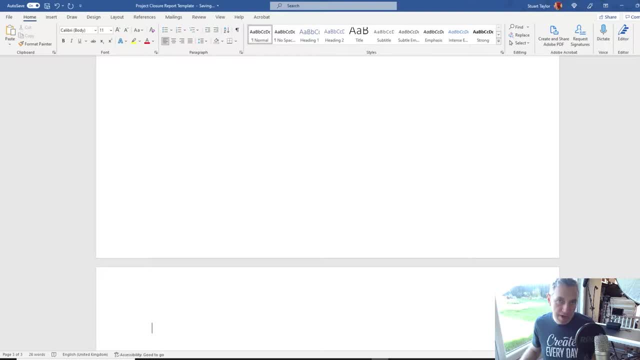 Here's what it looks like. Sorry, Sorry, All right itself. the first item we want to put in here is the project manager report, so we get a heading heading one, sorry, and we put the title project managers report. I'm just gonna put a note here to summarize the project's performance from: 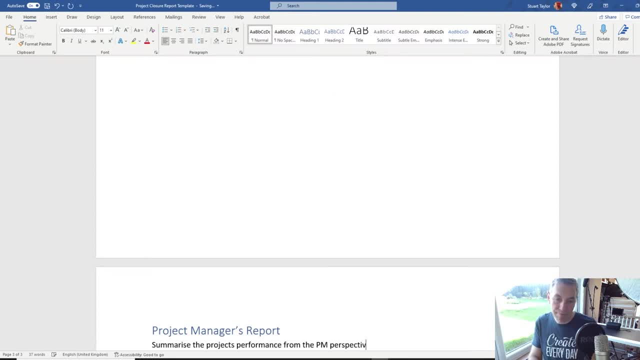 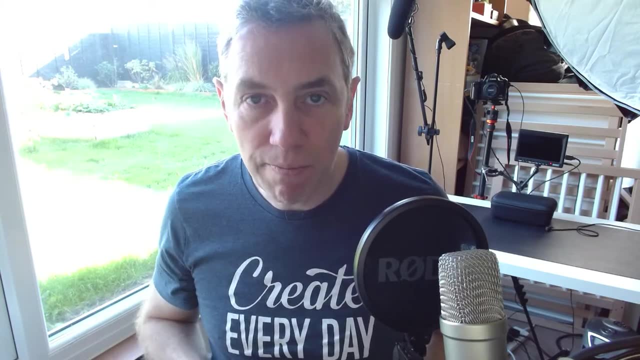 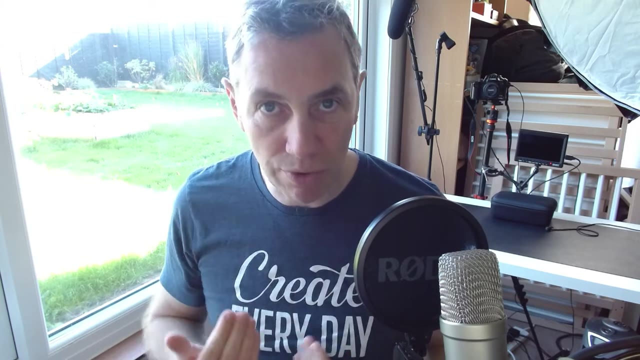 the PM perspective when you actually start filling out this report with actual content. you might want to come back to the project managers report last. if you complete the other sections of the report first, what will happen is you'll have those ideas and those thoughts at the front of your mind and you'll be 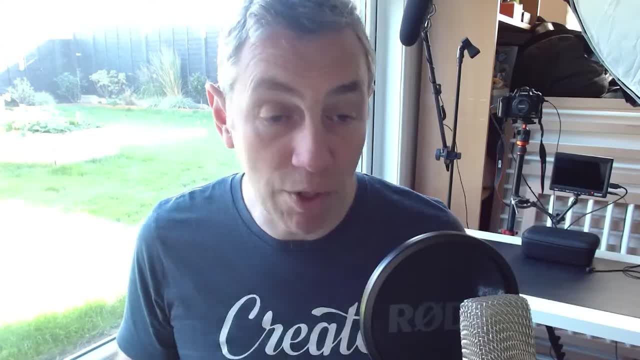 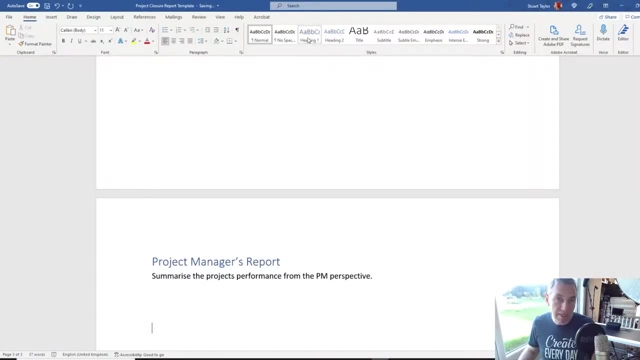 able to come back and write this project managers report a lot more easily. if you do the project managers report first, you might find you end up having to come back and tweak it and amend it. next part we're going to do is the review of the business case. 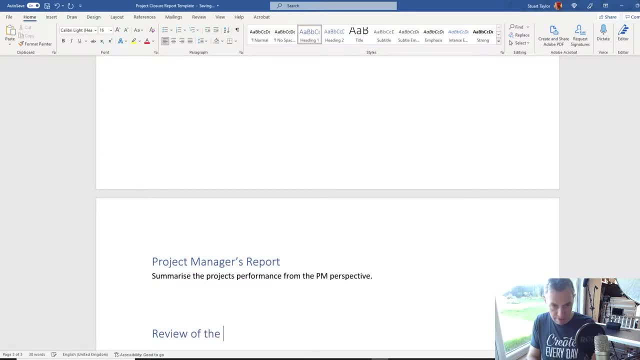 so we put a header in again, and here you might want to put some statements around whether you've delivered the benefits that were expected, if there any other benefits to be expected after the project is closed. the key thing to keep in mind here is you're actually doing a comparison with the original business case and 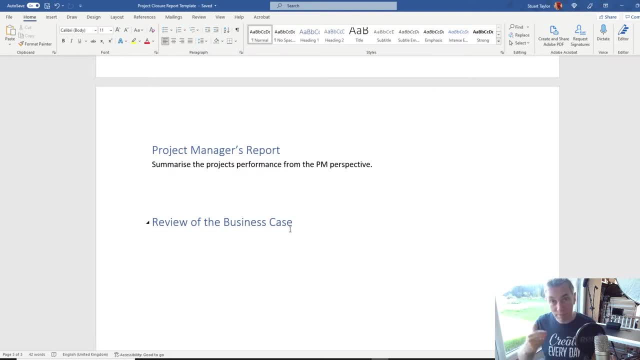 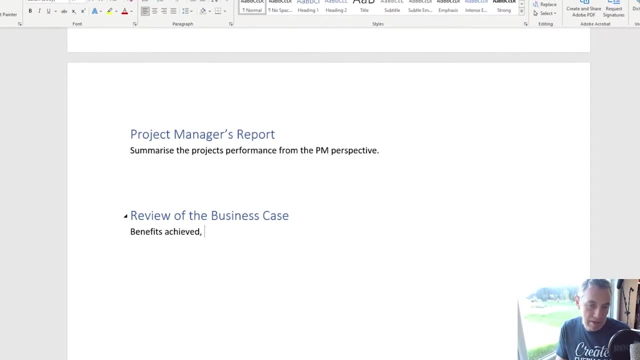 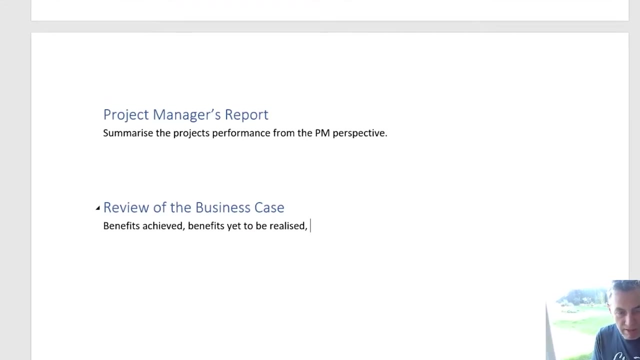 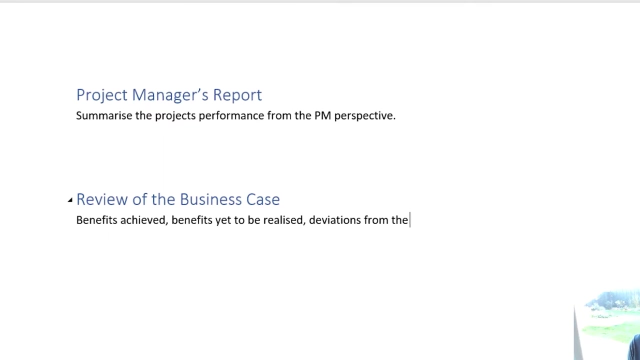 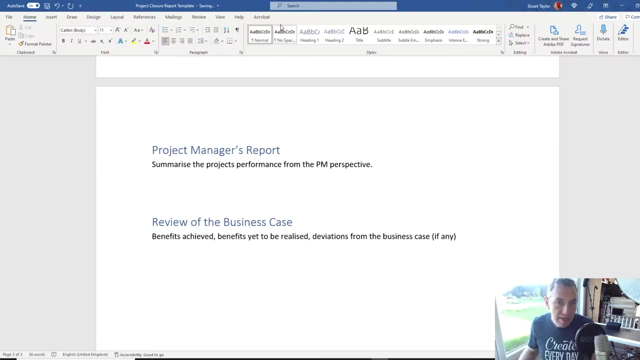 essentially looking back and saying: this is what we expected to do. this is what we did. I'll just put a note here that this will cover benefits achieved, benefits yet to be realized, and we'll include some deviations from the business case, If Any. the next section is the review of objectives, so we'll put another header in. 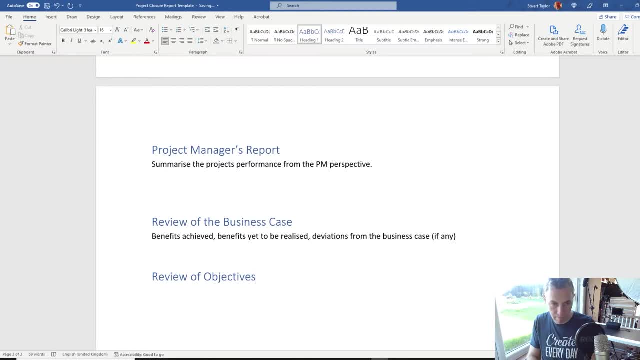 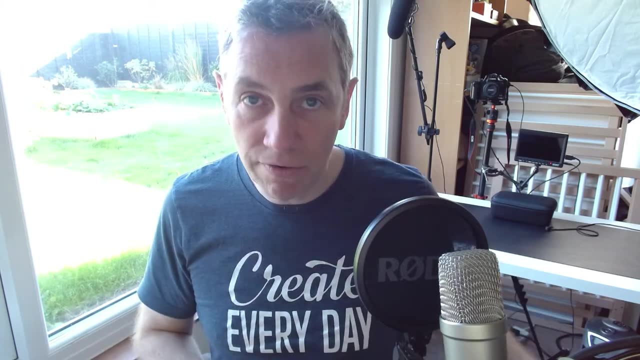 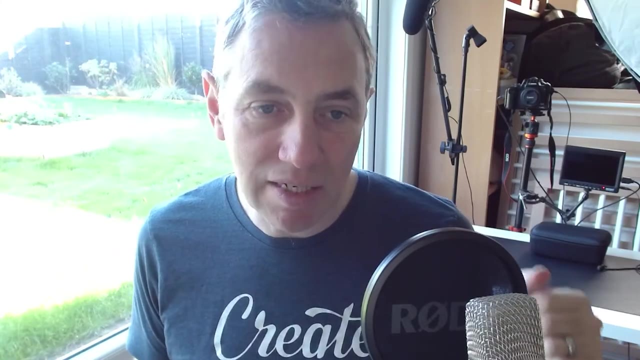 again, there's a lot of comparison going on in this part with the business case and other earlier estimations from the start of the project. to make it as easy as possible for you to get this report created quickly, i'm going to create a table that you can pretty much replicate, which will compare. 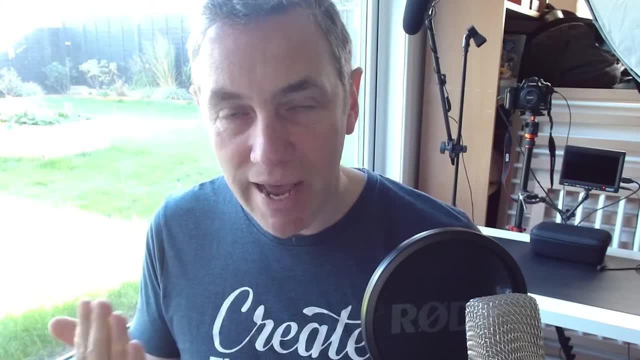 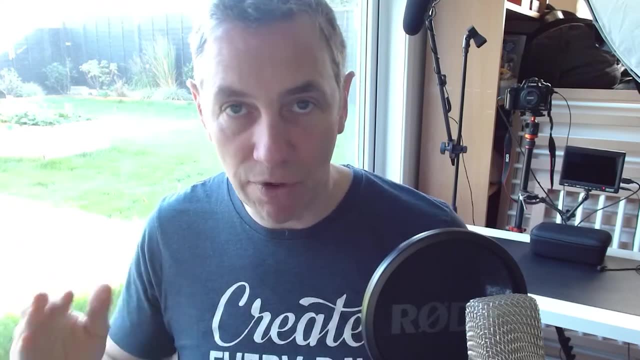 the original estimation and the final outcome and i'll include a section on there as well. there'll be a column that's going to look at the impact of any change requests that have altered things as the project's gone on. so when we get to the section with the key milestones, if you find that something's- 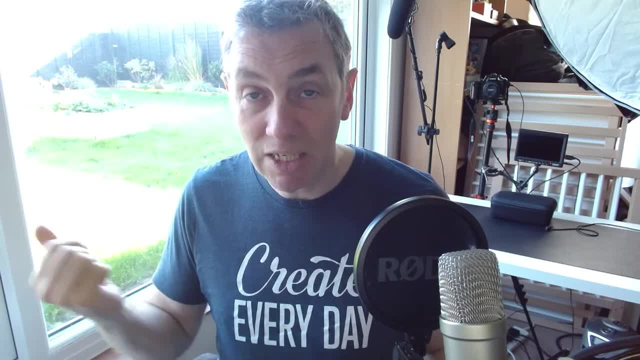 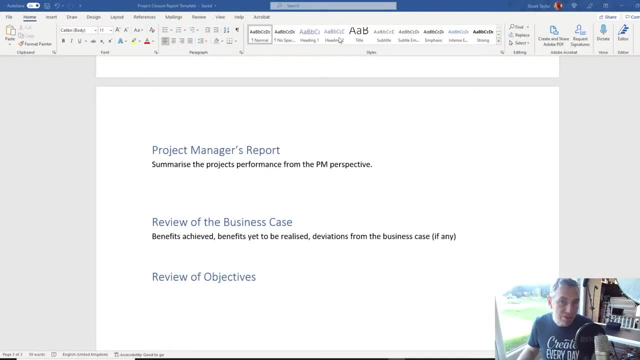 been delivered later than expected. if there was a change request that explained that and will give context to that story, then it's useful to have that linked in. okay, we're going to go to heading two now, which will create a subheading. let's start off with costs. let's insert a table by going to: 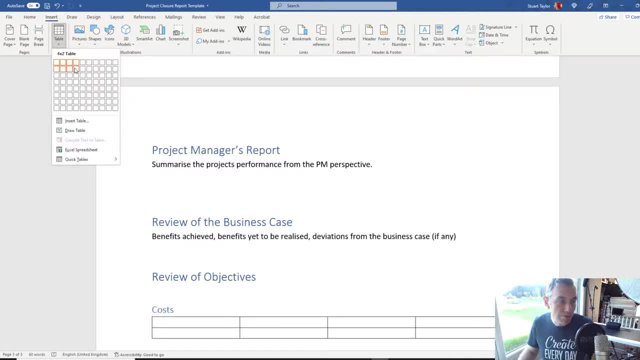 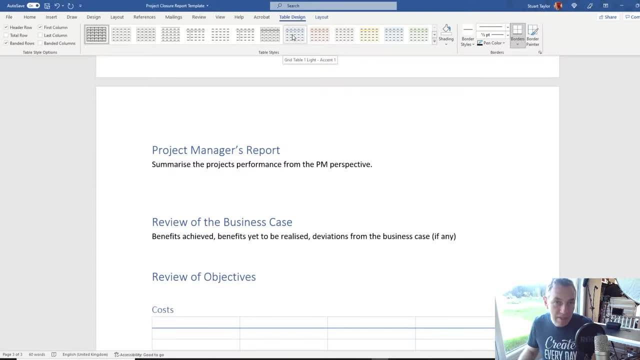 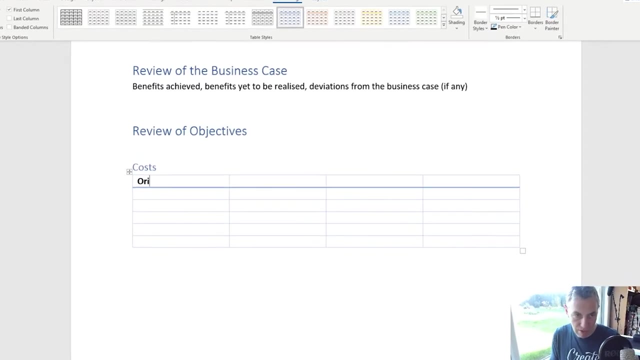 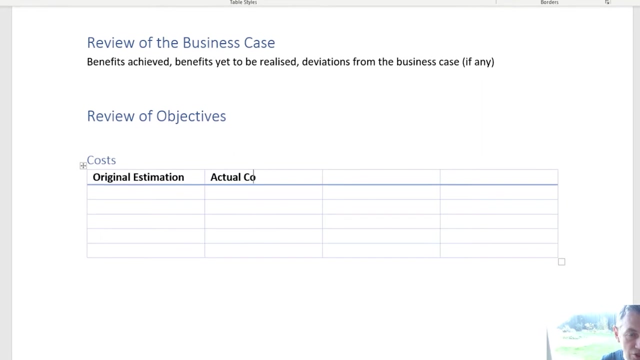 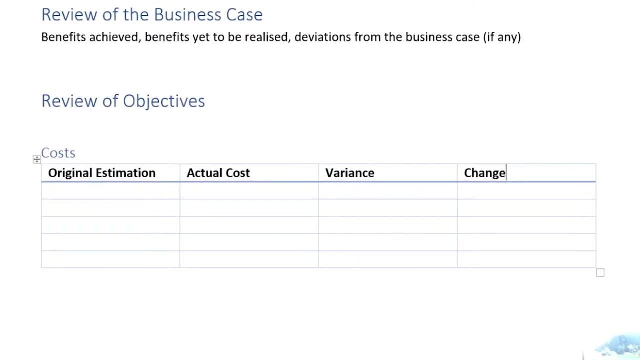 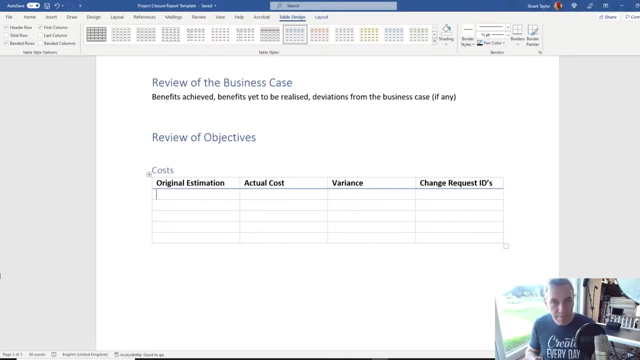 insert table, table, table, table, table. and this time we're going to put four columns and give it a few rows and we'll select the same table design that we used earlier. and here we're going to put original estimation, actual cost variance. this is our much it cost. whilst we're figuring out how we're going to do the project, this is how much it cost. 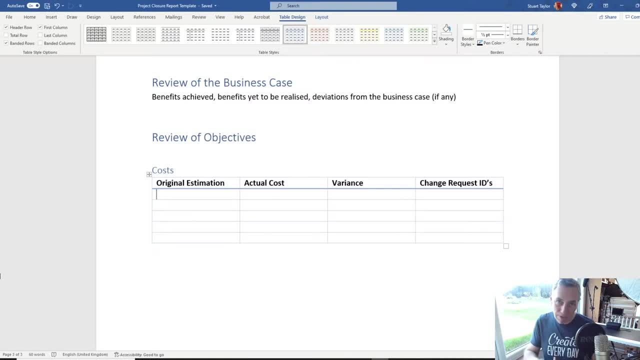 whilst we're planning and designing it, this is how much it cost when we're building it, this is how much it cost when we're testing it, and so on. Or you could do it a different way, you can go by. this is internal resource cost. this is external resource cost, this is suppliers and things and tools, and 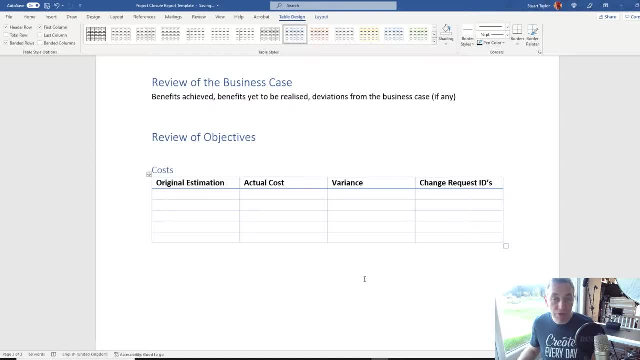 materials. however you want to put it, it's up to you. If you do decide to go into more detail than just having a single line entry, make sure to add a total row so that you can show what the total original estimation was, what the total actual cost is and what the total variance is. 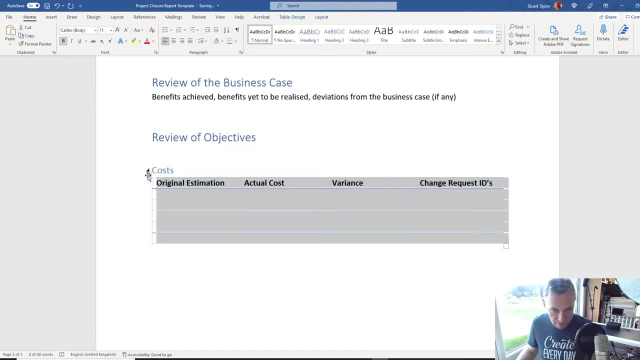 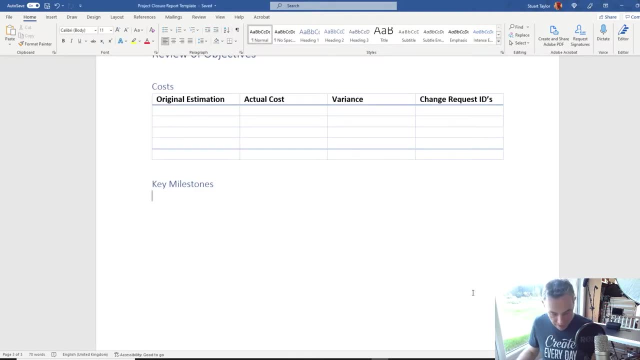 Okay, I'm now going to copy this table. it's going to be useful. Now we're going to add another heading called key milestones. Okay, now we're going to paste that table in that we copied earlier. We're going to select the first of the columns and right click on the table and go to 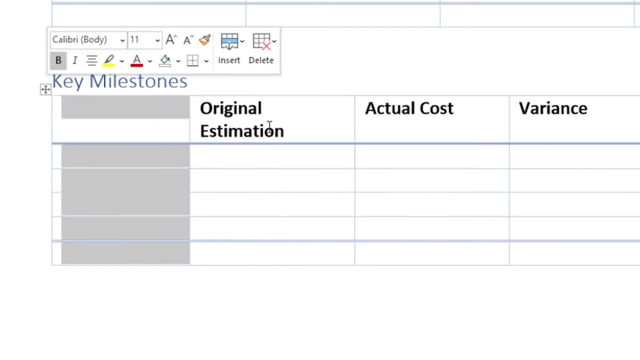 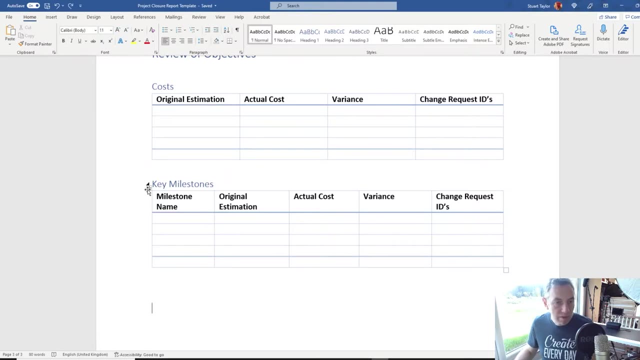 insert Left. Insert left. We'll put milestone name here. Okay, so we can select the table and go to table design and get rid of that total row. we don't need it on here And we'll change original estimation to target date. 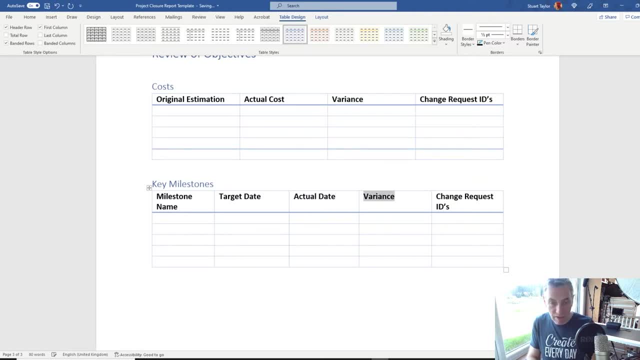 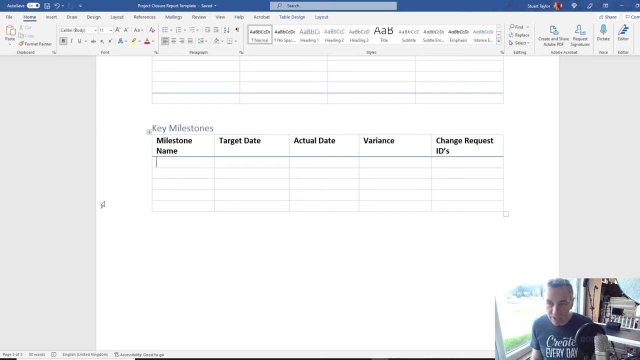 Change this one to actual date Variance which you can record in days, weeks, months, Even if you're in that situation- And again, we keep the change request ids on here- When you're populating this section, make sure to include key events such as the end of stages. 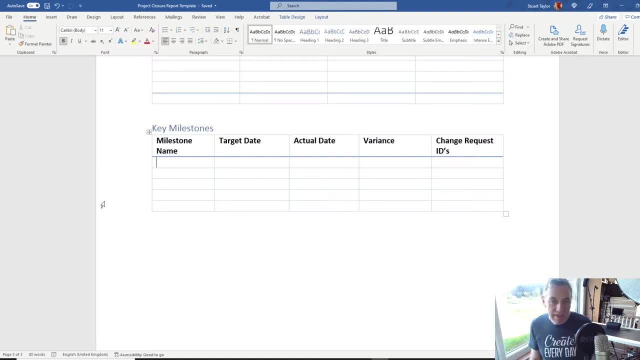 go live dates, release dates, handover dates and so on. Okay, let's put another subheading in Select heading two. We'll call this one scope. Again, we can paste that table in again if we choose to, or we can just write a new one. For this one we're going to put whole. 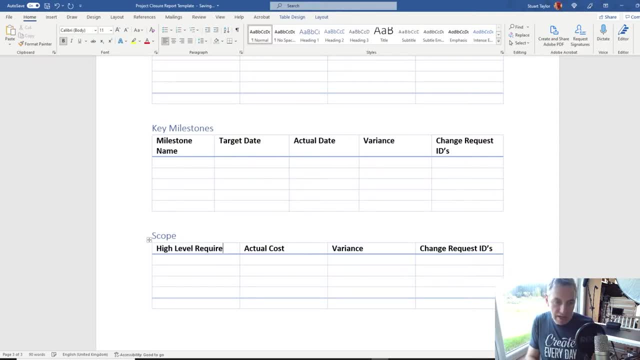 high level requirement. You can go into a lot more detail, but you should have a requirements document that will have kept track of all of this. In this one, we'll put a simple statement of whether it's been achieved or not. We'll leave variance on here so you can explain the nature. 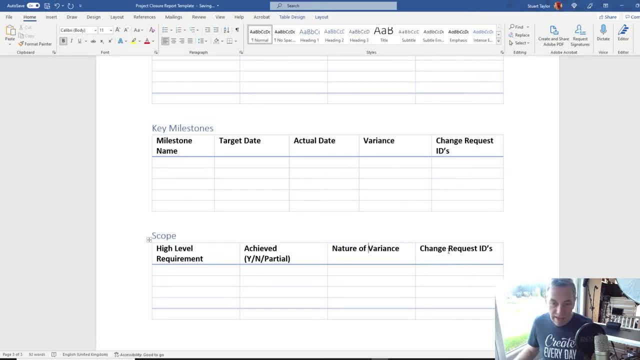 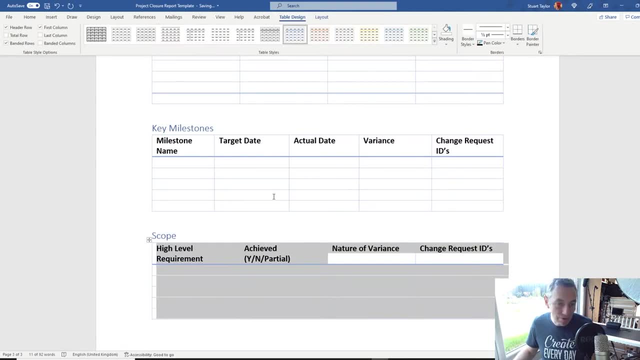 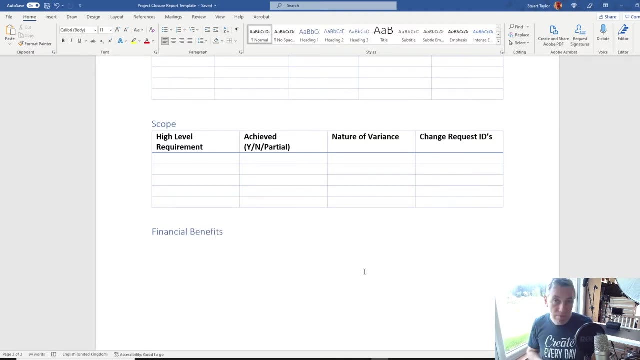 of any variance that has occurred And again, we'll leave a section here for the change requests. Again, highlight the table- It's a table design- and get rid of that total row. Next we're going to put a section for financial benefits. You've already had a section where you've talked a little bit about benefits. 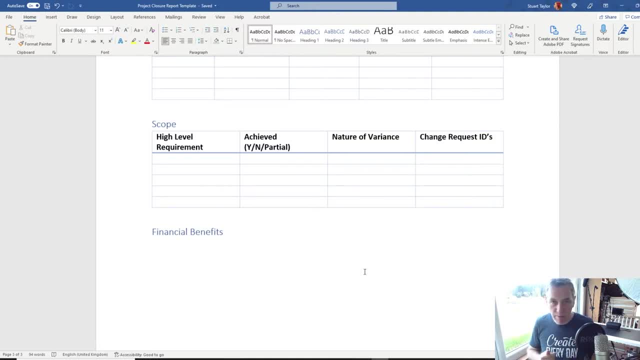 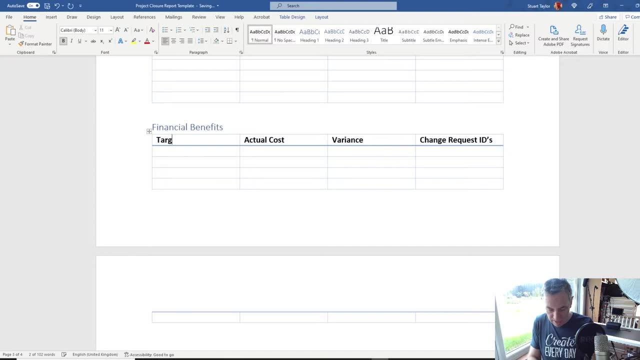 But what we're going to do in this part is actually break that down into a little bit more granular detail. Okay, I've pasted the table in from earlier and I'm going to add target benefit. We'll leave the variance and the change requests Underneath this one, though we'll put a note. 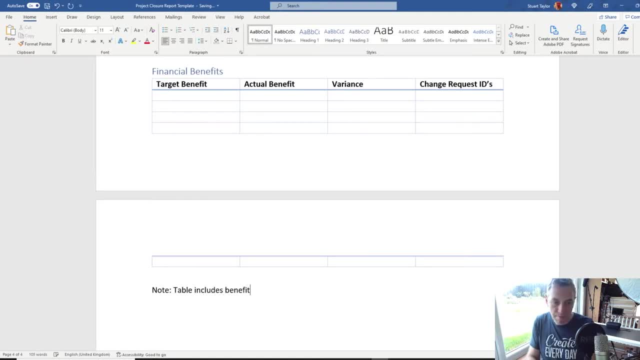 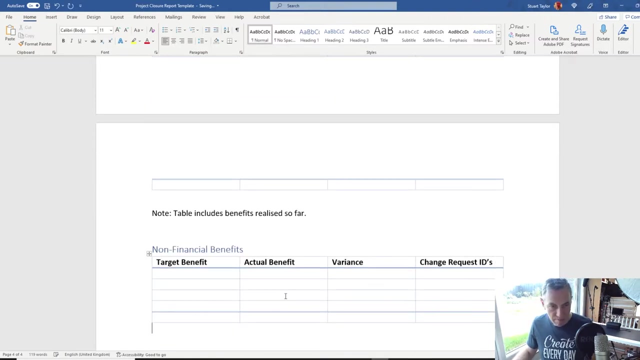 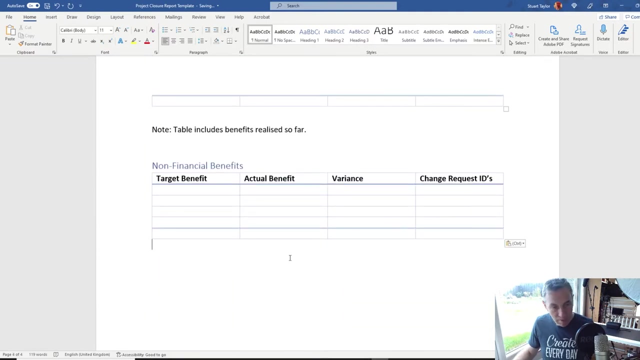 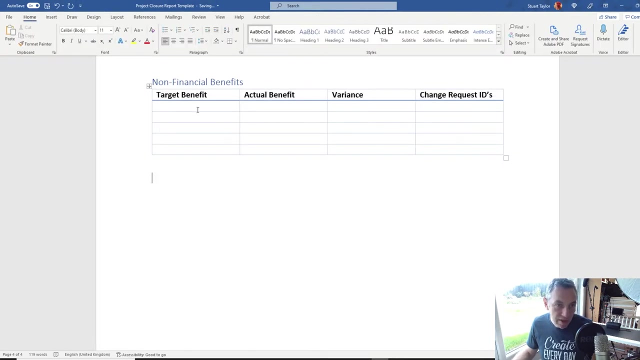 table includes benefits realized so far. Now we'll select heading 2 again and we'll add a section called non-financial benefits. This time we can just have a straight copy of this table. By the way, I should mention that on the financial one I did leave the total row, so on this table I'm 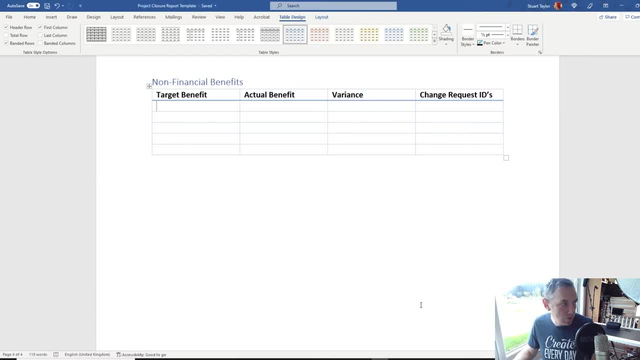 just going to highlight the table again. go to table design and get rid of the total row. Again, you can put a description in here. It is a little different, though, from the financials. in this case, you might be saying: something's going faster, something's improved its quality. 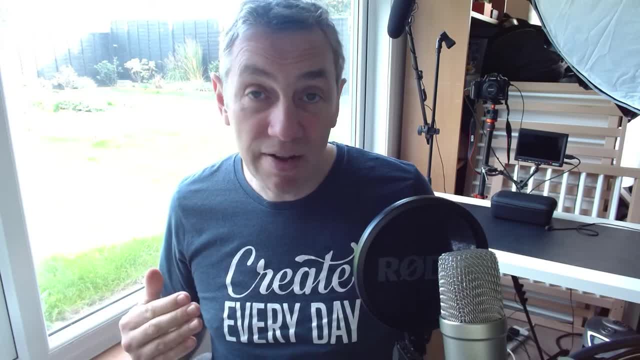 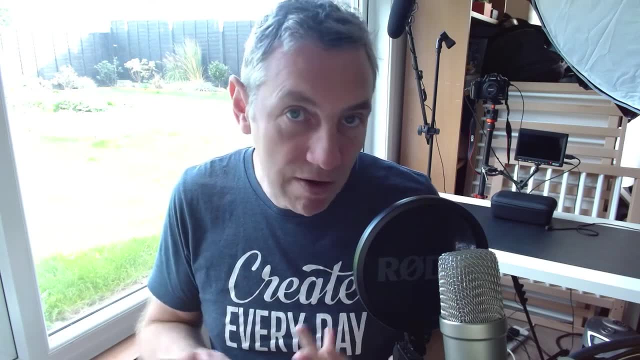 The content in the non-financial benefits section types. The size of the expansion 왼 the department shufa vade table is going to vary a lot depending on the project. it could be that you made things faster, better, better customer experience, so on. it could be any kind of. 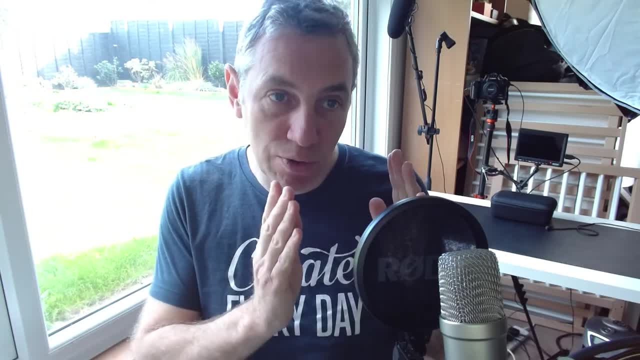 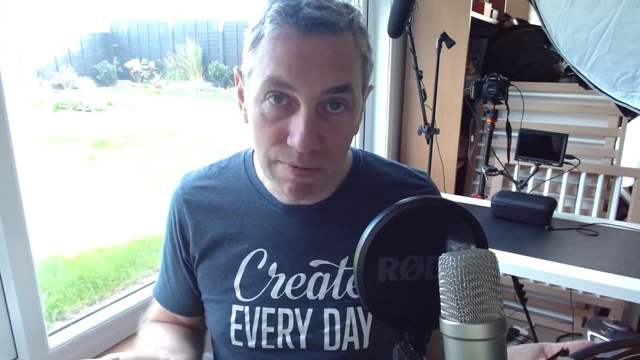 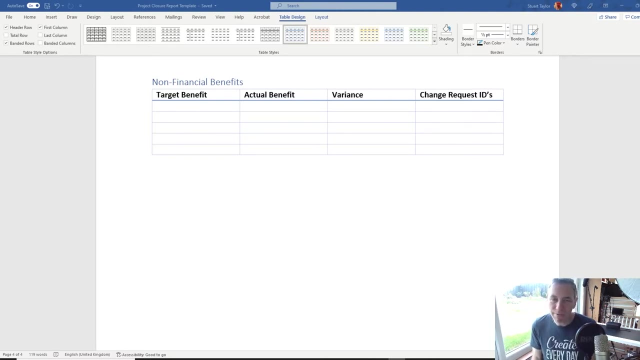 measure. so hopefully, if you log your target benefits that you had from the start of the project against your actual, you can explain the variance. it still works. there is an argument to say that quality and risk should appear on here as well. I've typically found that they're not actually really wanted in. 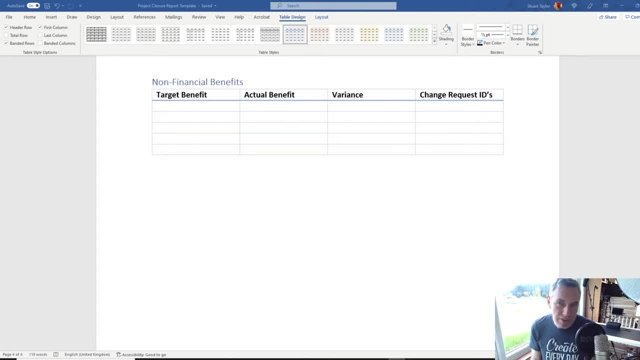 many organizations quality gets covered a little bit later on a risk. people only really seem to care about that at this stage. if there are open risks or risks, they're being transferred to the organization. so that will be addressed a little bit later on as well. so now we're going to click into the page and add: 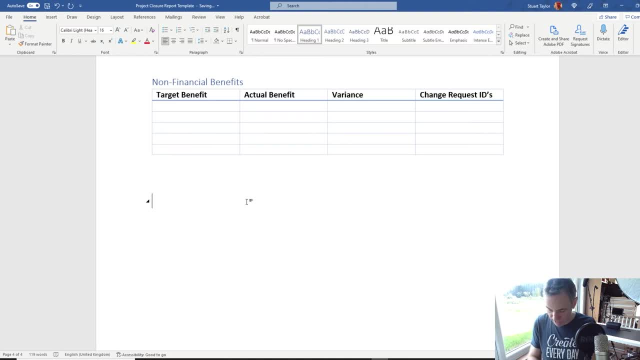 heading one and this will be review of the project product. so we go to heading two again to create a subheading and we put quality and in this section you can add details of quality expectations and whether they were met. I'll also put explain any deviations. okay, we'll put heading two. 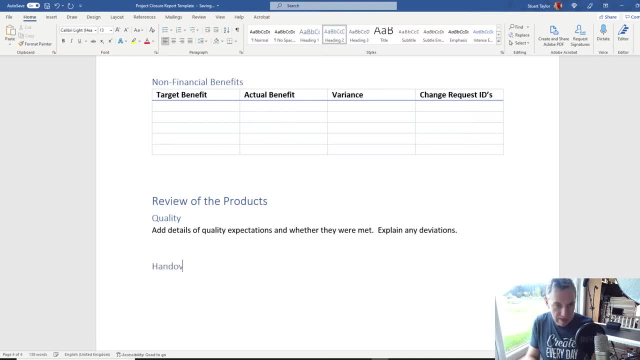 on here again and call this handover of products, and here we're going to include a statement from the business owner. this will just be a straight copy of any email that they've sent across to you, where they've confirmed receipt of the products and they give their feedback on: yes, it's a good product and yes, it's a. 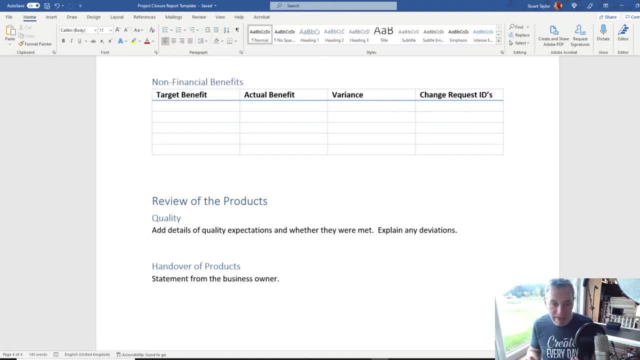 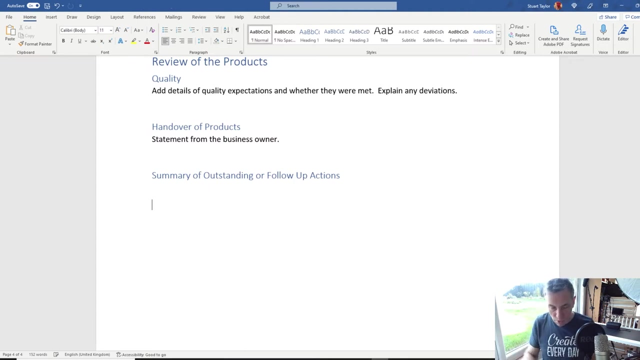 bit of purpose, or no, it's not. we've got some outstanding actions, speaking of which, then we'll put a heading two and summary of outstanding or follow-up actions. now what you could do here is you can either write a narrative around this. what I actually prefer to do is to insert another table. you'll be shocked. 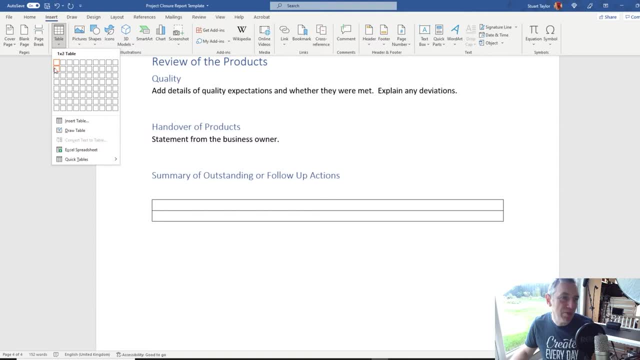 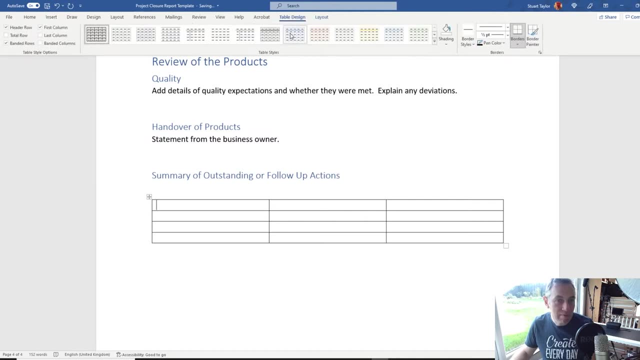 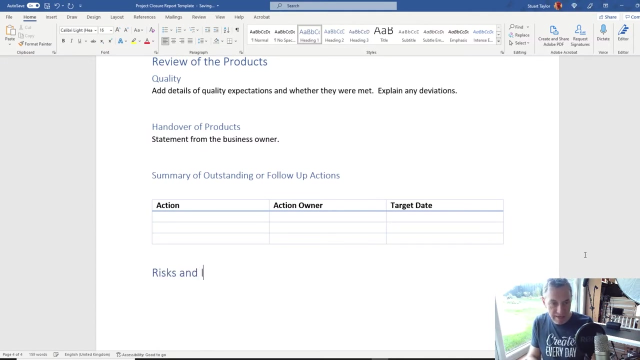 to hear- which will have enough columns to include the action itself, its owner and its target date. I'll go to the table design then. so same format we've used before: action, action, owner, target date. okay, then we go to heading one: risks and issues. we're going to put a simple table in this section. it's going to: 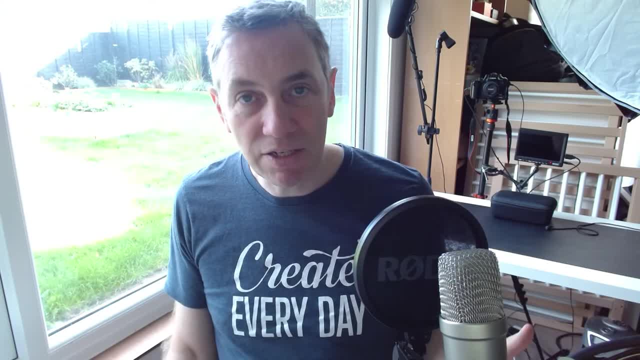 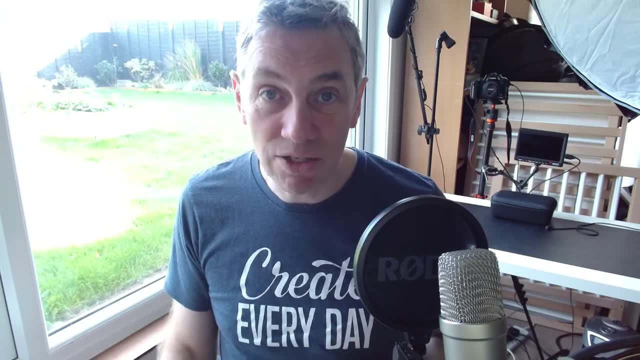 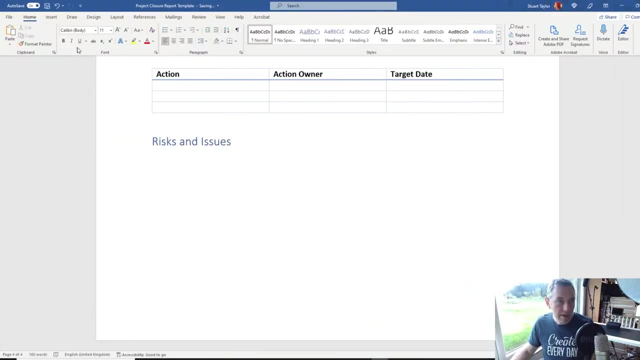 explain any open risks and issues they've had to transfer, either because time ran out, they couldn't be completed as part of the project, or because the project that itself has created new risks and issues that have been handed across to the business along with the outputs of the project. okay, so let's go. 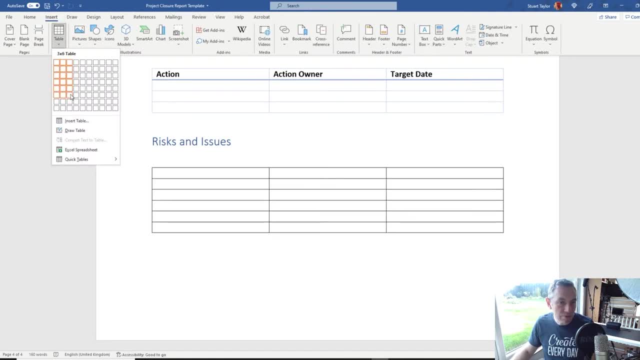 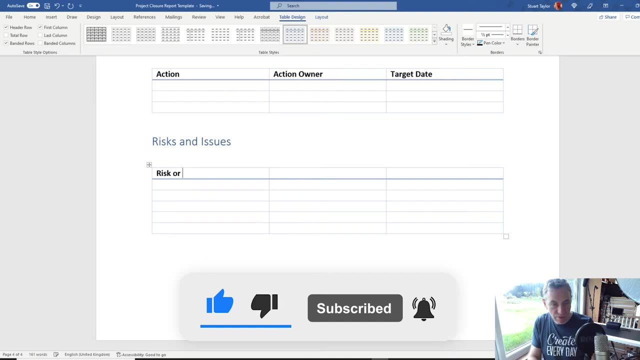 to insert select table. three columns select the same table design that we've used earlier. risk issue: new owner and date transferred. don't forget you don't get to just chuck this over the fence at the new owner. they need to receive it, they need to be the right person for it and they need to confirm that they're. 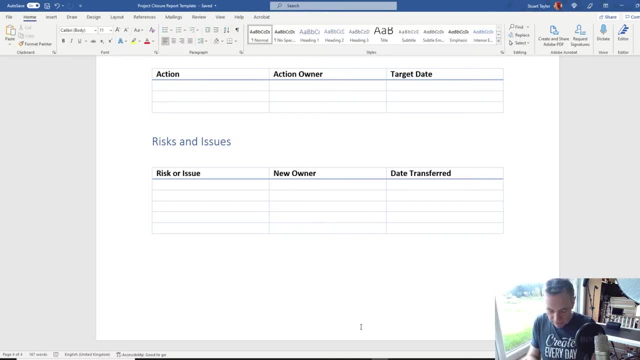 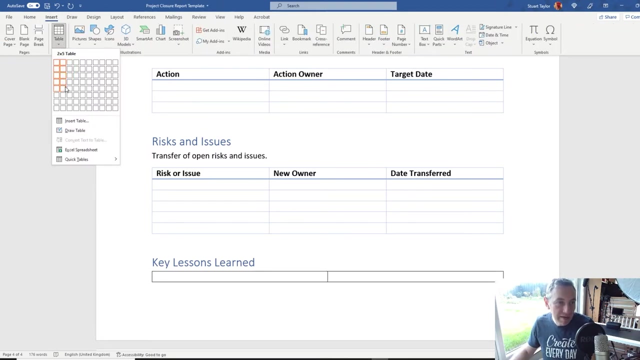 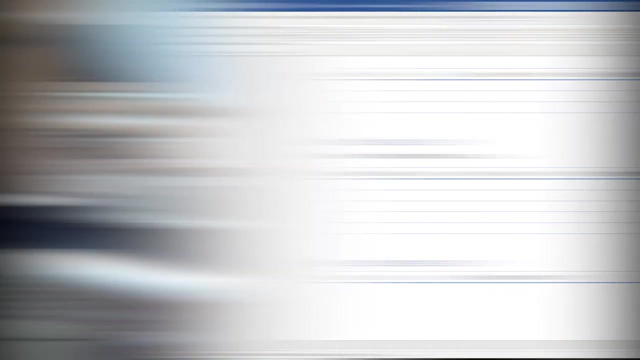 going to take care of it. going forwards, I'm just gonna put a little narrative at the top just in case we ever forget. okay, go back to heading one again for the new section, and we're gonna call this key lessons learned. and again we're gonna insert a simple table. again we'll call this lesson recommendation. I should 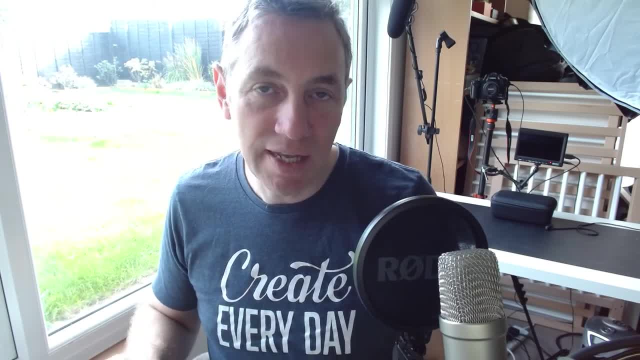 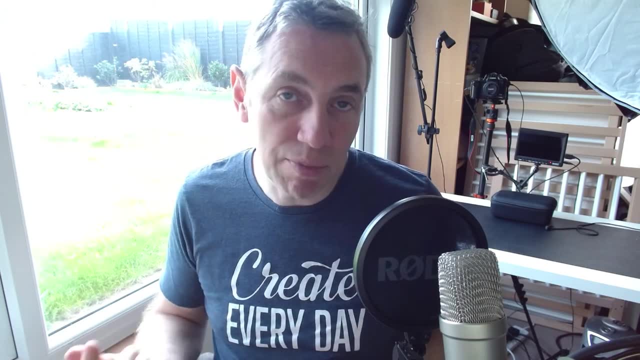 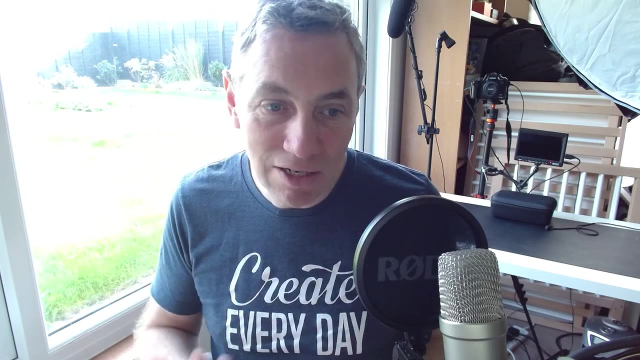 add, whilst we're doing this, we're only putting in the key lessons learned here. there should be a full lessons learned library somewhere else in your records, so you just need to have a hyperlink at the end of this table pointing back to wherever that exists. on that basis, you don't need to replicate the entire contents of the lessons into. 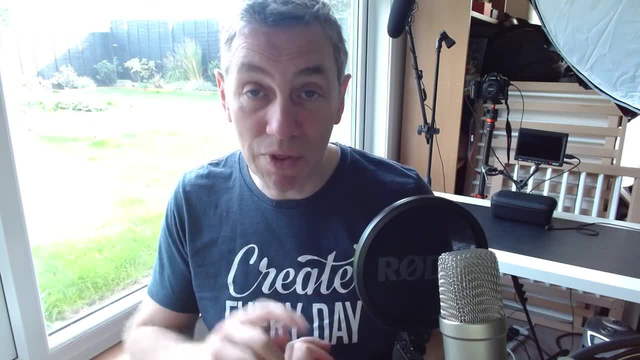 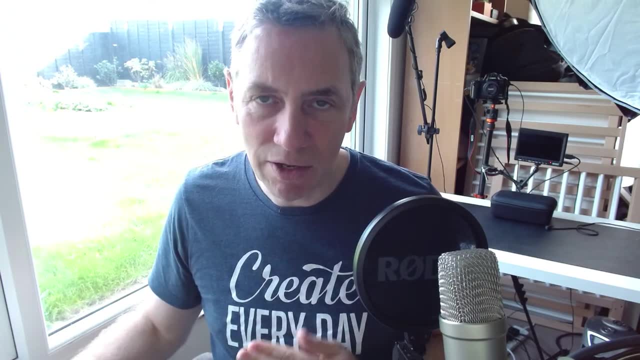 this table. just make sure that you include a fairly high level description of what the lesson is, what the recommendation from that lesson is, and I'm gonna add some more content onto this as well. you don't need to do this, this is optional. I'm gonna add. 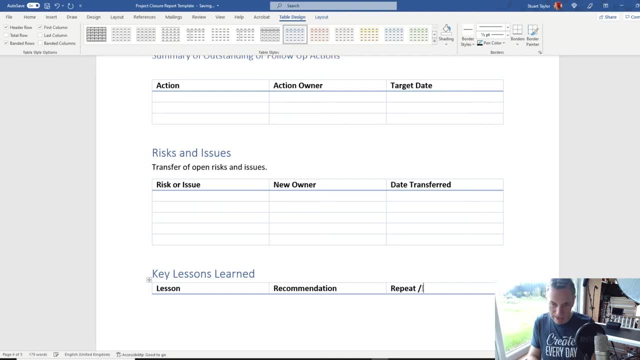 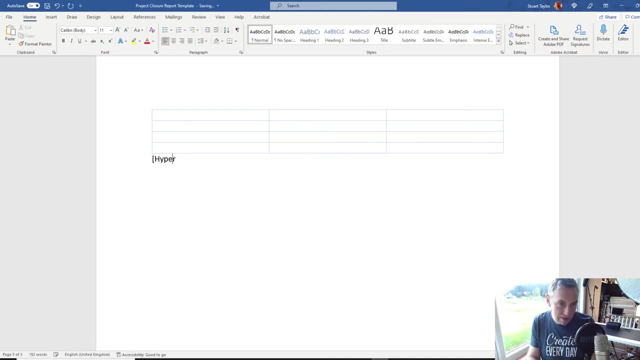 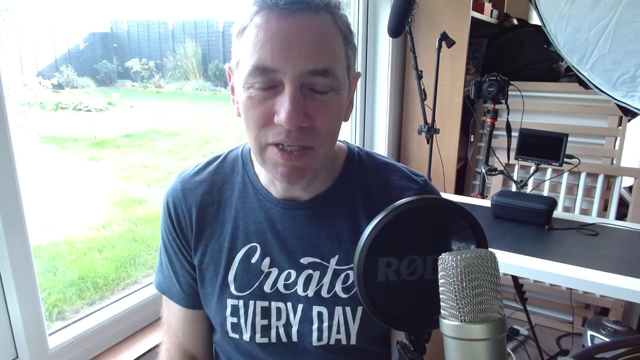 repeat and avoid. underneath the table. I'm gonna make a recommendation to add a hyperlink to full lessons log. okay, we're nearly at the end and what we've got so far would usually be sufficient for most places, but I'm going to include a section that sometimes gets overlooked. we're gonna make sure that it's in the 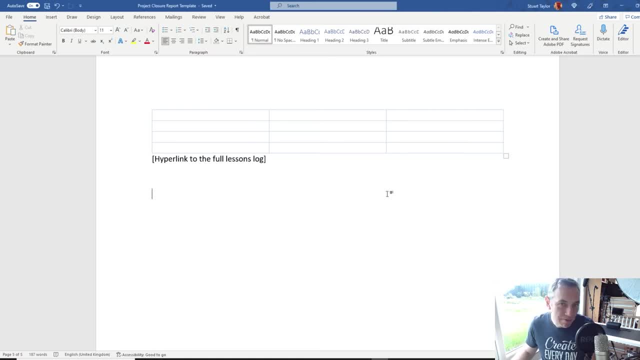 course, and then click on add, then we're going to add a section to this. that's fine, as that's what we do for this one, and what I suggest is we add a section here. that's gonna go from content to content. so if you're working on an 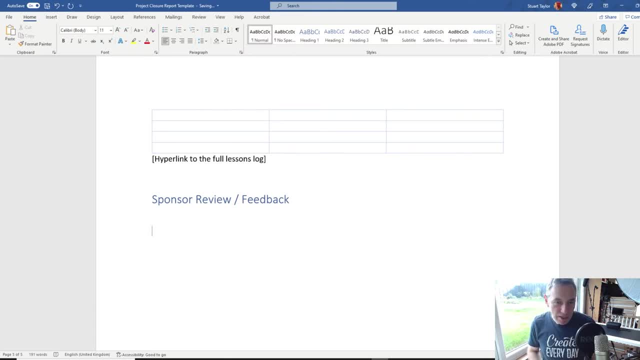 implementation of the lesson for a lay writer, for example, and if you're playing a game that's not a lay writer, then that's all you're doing is you're going to add that section here. I'm going to add a section called review, and sponsor to do is to give their impressions at this moment in time of how the project has gone. 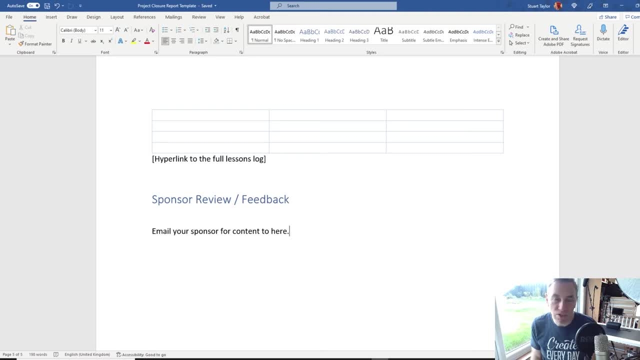 if things have gone particularly well, if you've overcome significant challenges or if you've over performed and over achieved, you want that to be called out in here. if things could have been done better from their perspective, it's worth adding here as well. don't forget the purpose of. 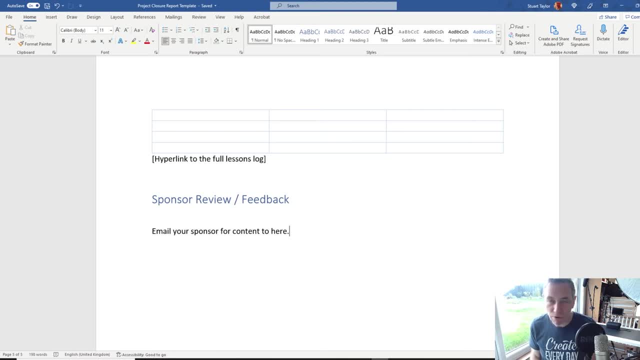 this report is to help the organization and future project managers to learn as they deliver their projects as well. so if there's a lesson to be learned just from the sponsor's perspective here, it's worth collecting it. don't forget we can learn just as much from things that went wrong.